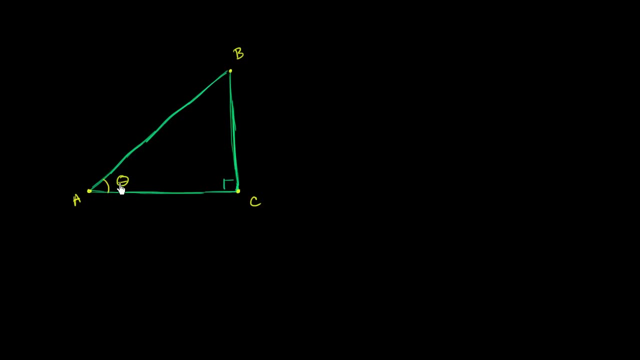 I guess we could call it angle A. let's say it's equal to theta. If this is equal to theta, if its measure is equal to theta degrees, say what is the measure of angle B going to be? Well, the thing that will jump out at you. 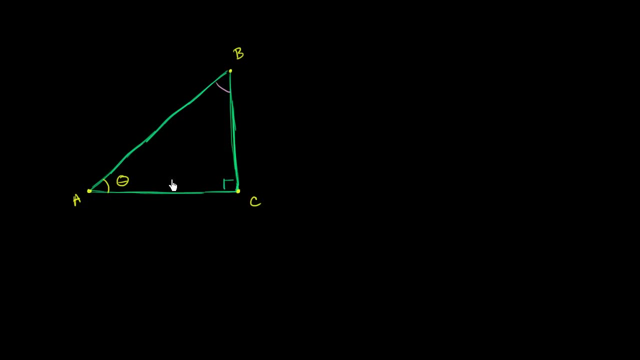 and we've looked at this in other problems- is the sum of the angles of a triangle are going to be 180 degrees, And this one right over here it's a right triangle, So this right angle takes up 90 of those 180 degrees. 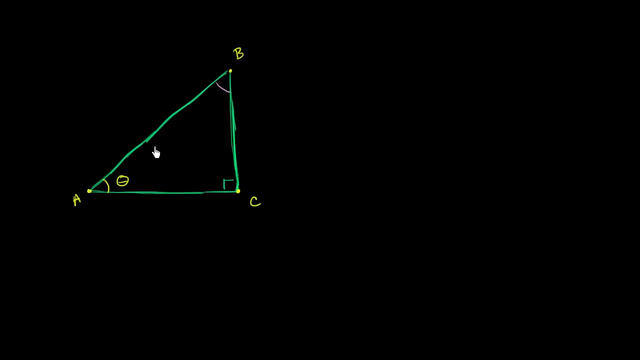 so you have 90 degrees left, So these two are going to have to add up to 90 degrees. This one and this one, angle A and angle B, are going to be theta. They're going to be complements of each other. 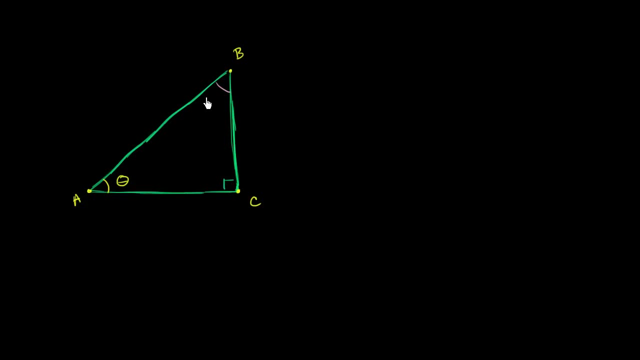 They're going to be complementary. Or another way of thinking about it is: B could be written as 90 minus theta. If you add theta to 90 minus theta, you're going to get. you're going to get. or theta to 90 degrees minus theta. 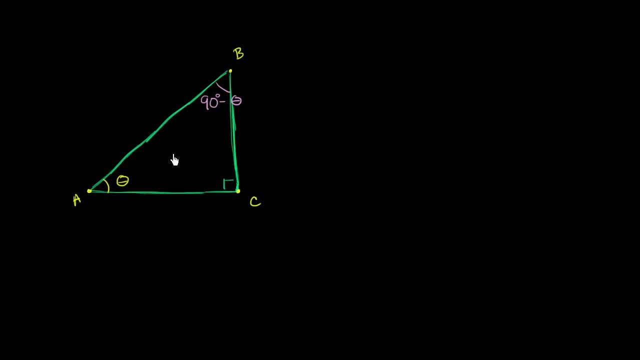 you're going to get 90 degrees. Now why is this interesting? Well, let's think about what the sine of theta is equal to. of theta is equal to. Sine is opposite over hypotenuse. The opposite side is BC. 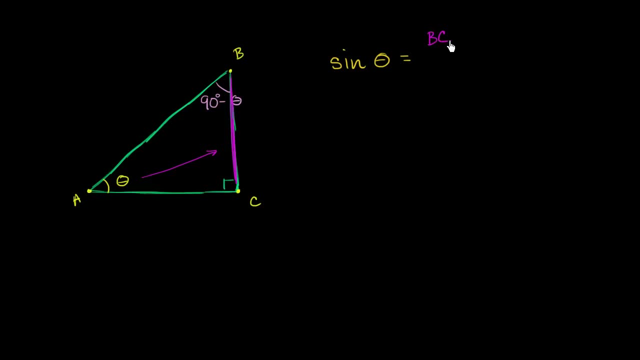 So this is going to be the length of BC over the hypotenuse. The hypotenuse is side AB, So the length of BC over the length of AB. Now, what is that ratio if we were to look at this angle right over here. 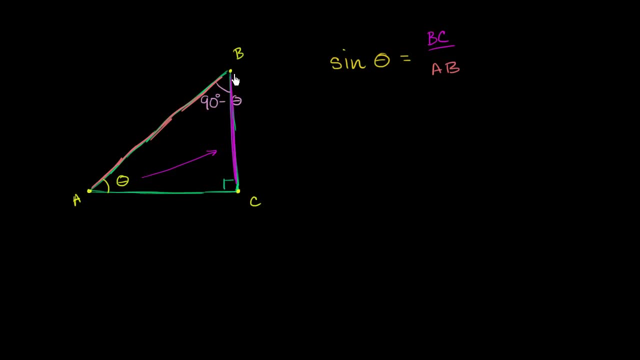 Well, for angle B, BC is the adjacent side and AB is the hypotenuse. From angle B's perspective, this is the adjacent over the hypotenuse. Now, what trig ratio is adjacent over hypotenuse? Well, that's cosine. 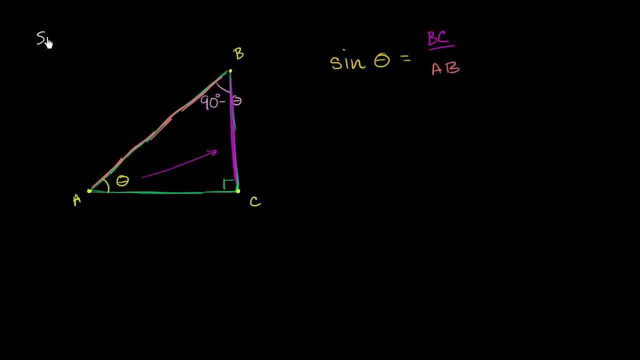 So k? toa, Let me write that down. Sine doesn't hurt. Sine is opposite over hypotenuse. We see that right over there Cosine is adjacent over hypotenuse. k And toa tangent is opposite over adjacent. 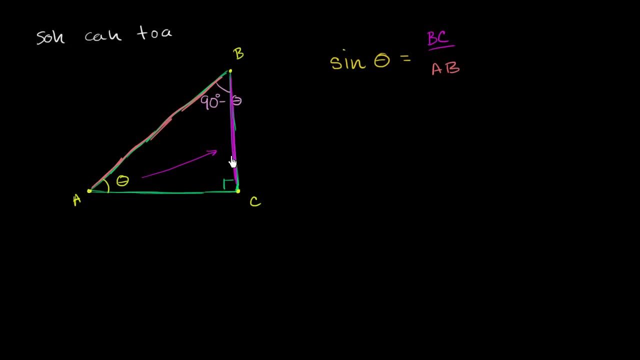 So from this angle's perspective, taking the length of BC, which BC is its adjacent side and the hypotenuse is still AB. So from this angle's perspective, this is adjacent over hypotenuse, Or another way of thinking about it is the cosine of this angle. 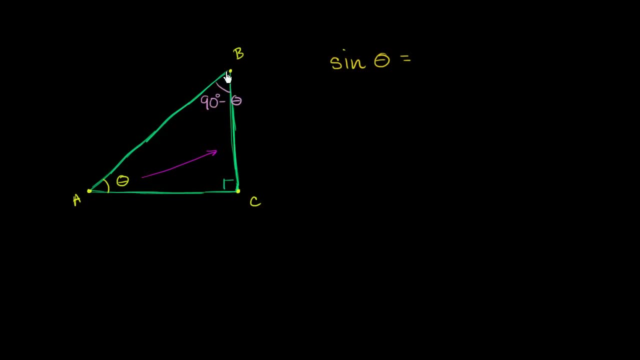 Sine is opposite over hypotenuse. Sine is opposite over hypotenuse. The opposite side is BC. So this is going to be the length of BC over the hypotenuse. The hypotenuse is side AB. So the length of BC over the length of AB. 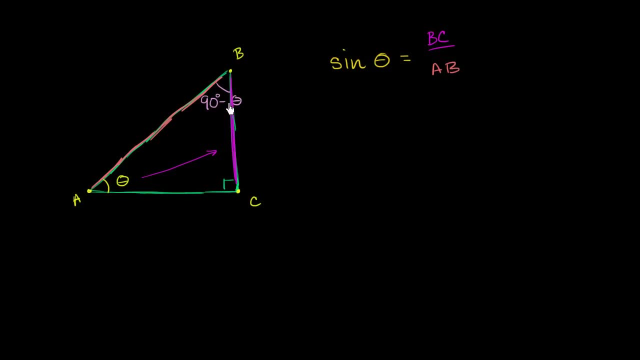 Over the length of AB. Now, what is that ratio? if we were to look at this angle right over here? Well, for angle B, BC is the adjacent side and AB is the hypotenuse. From angle B's perspective, this: 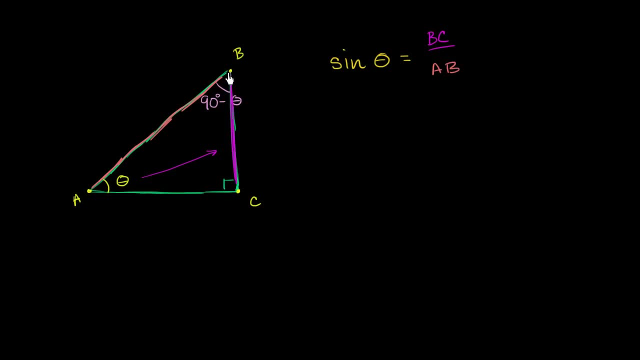 is the adjacent over the hypotenuse. Now, what trig ratio is adjacent over hypotenuse? Well, that's cosine. So k toa, let me write that down. Sine doesn't hurt, Sine is opposite over hypotenuse. 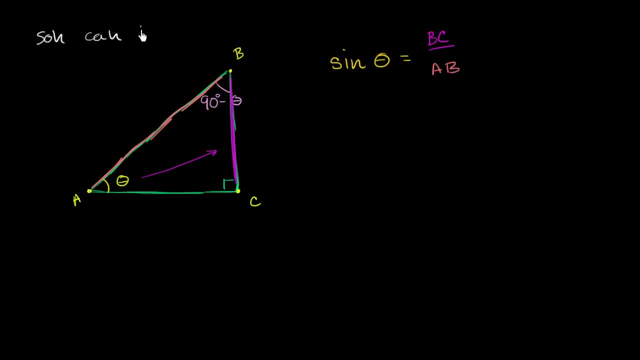 We see that right over there Cosine is adjacent over hypotenuse k And toa tangent is opposite over adjacent. So from this angle's perspective, taking the length of BC, which BC is its adjacent side and the hypotenuse, 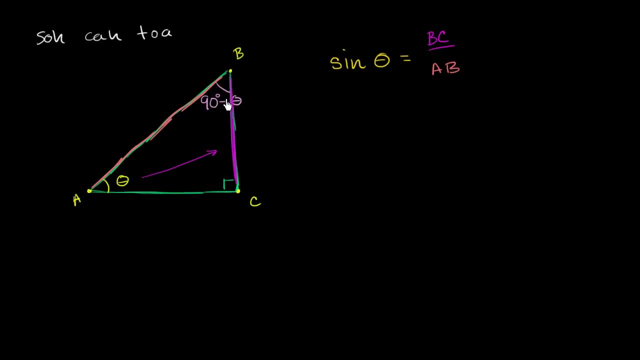 The hypotenuse is still AB. So from this angle's perspective this is adjacent over hypotenuse, Or another way of thinking about it, is the cosine of this angle. So that's going to be equal to the cosine of 90 degrees. 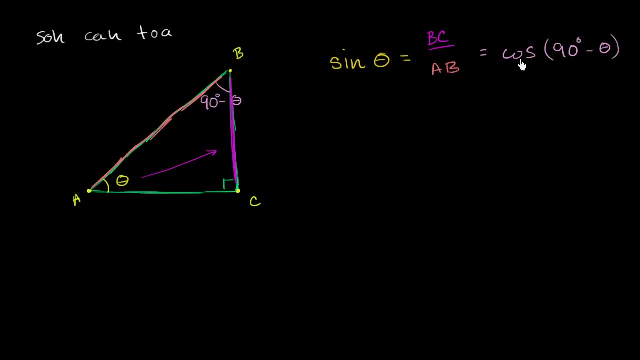 minus theta. That's a pretty neat relationship. The sine of an angle is equal to the cosine of its complement, So one way to think about it, the sine of- we could just pick any arbitrary angle. Let's say the sine of 60 degrees is. 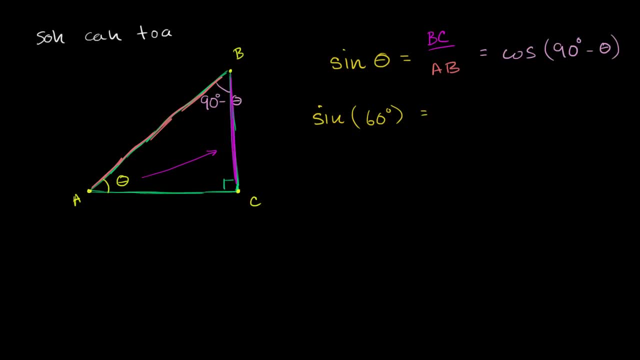 going to be equal to the cosine of what- And I encourage you to pause the video and think about it. Well, it's going to be the cosine of 90 minus 60. It's going to be the cosine of 30 degrees. 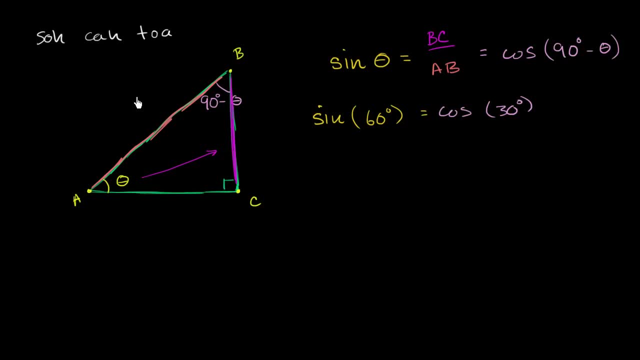 30 plus 60 is 90. And of course you could go the other way around. We could think about the cosine of theta. The cosine of theta is going to be equal to the adjacent side to theta. to angle A, I should say: